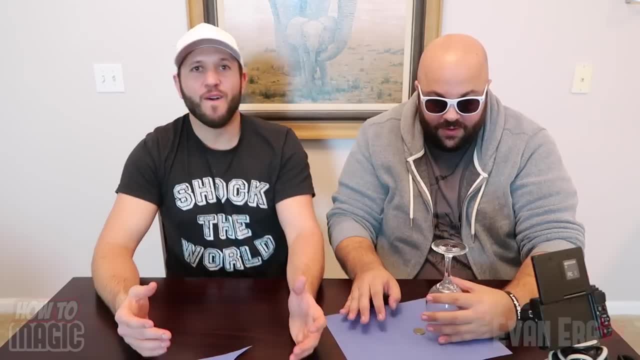 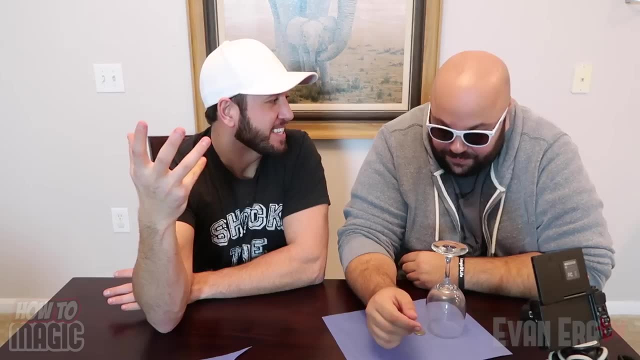 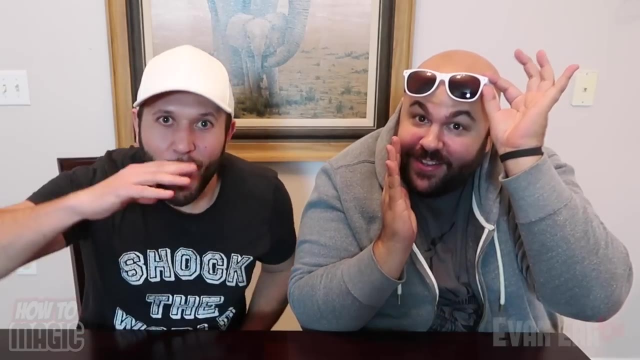 One more time. Whoa, You got to show us how to do it. man, You want to see what happened? Say it right now in the comments. How did you do it? Get ready, because Evan's about to reveal a secret. 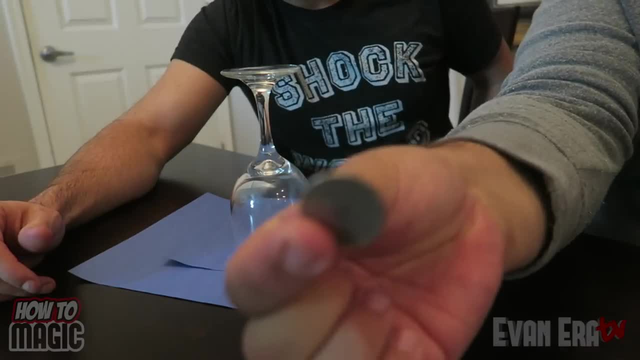 Okay, so all you need to perform this trick is a wine glass, a coin, some glue, a pair of scissors and a couple pieces of paper. Okay, so your first step is to take the cup and you're going to sit it down on the paper. 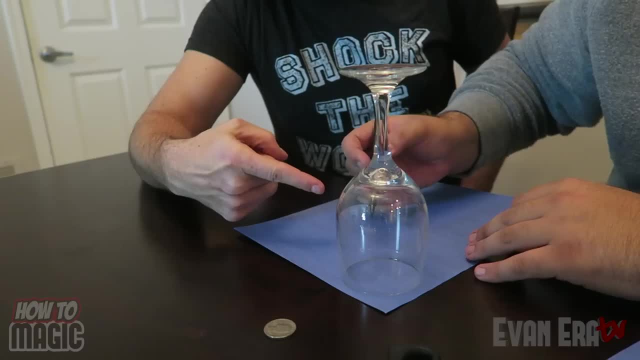 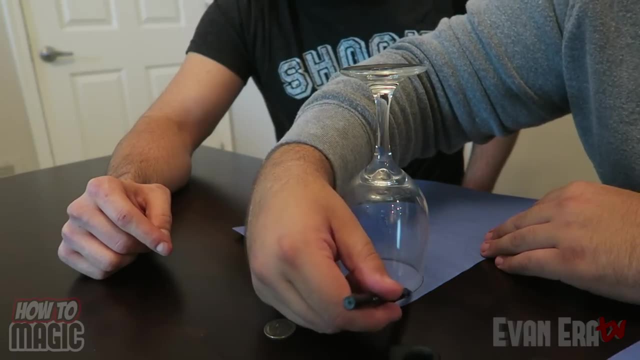 We're going to trace around the Wait, you need a pen too. You do need a pen. All right, I guess I forgot to mention that. You trace around the cup like this: This is just going to give you like a rough idea of what you need to cut out of the paper, and you're just going to cut this out. 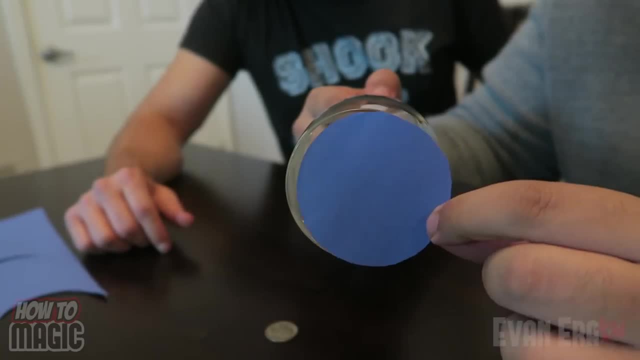 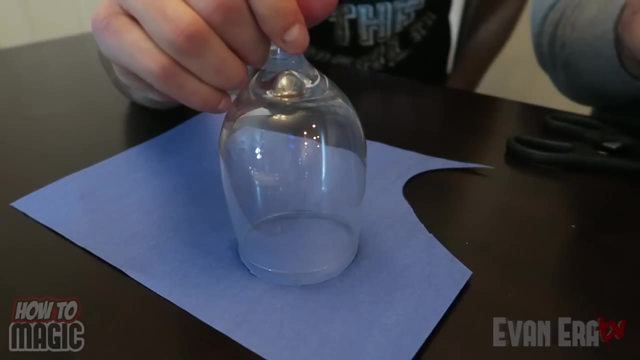 Okay. so now that you have your circle of paper cut out, you're going to glue that to the top of your wine glass. We're going to run a little bead of glue around the outside edge of it and press your cup down right on top. 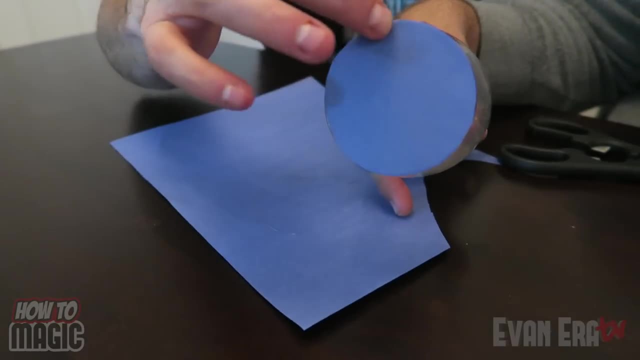 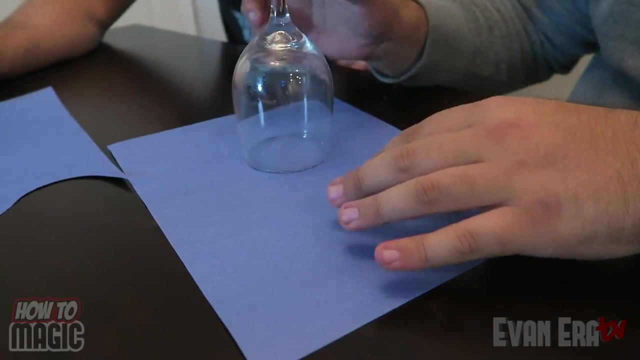 You really want to just push down around the rim. Do a good job like a good rim job here, as you push and make sure the glue and paper are stuck to the cup. So now, when you have the cup sitting on the paper, Whoa. 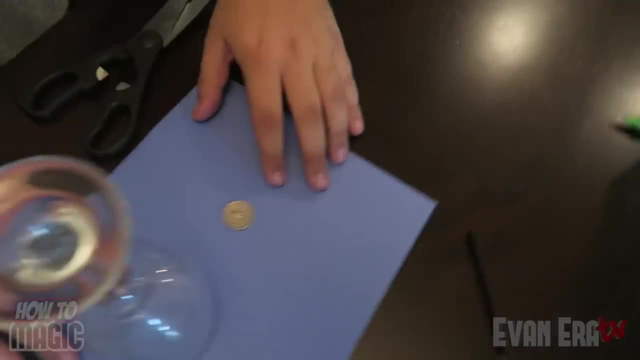 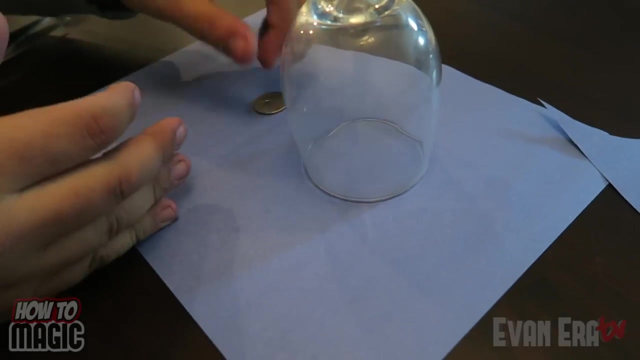 I can't tell. You can't Look at this angle. That's pretty cool, Holy crap. Now you can't tell that the paper is glued to the cup. It looks like your cup is just sitting on there. Wow, So now. 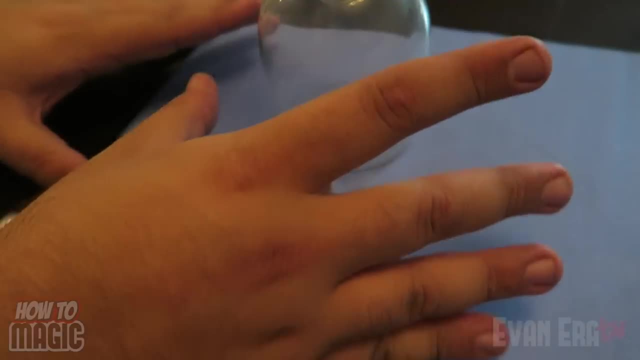 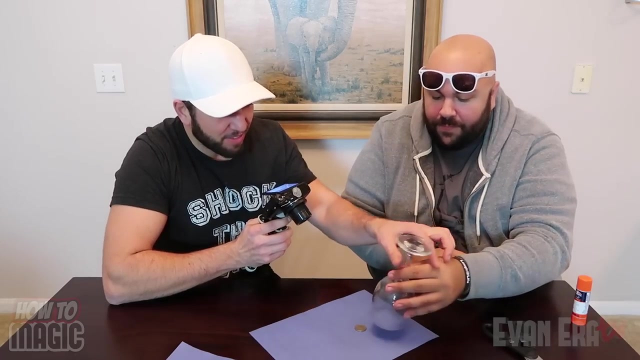 That's awesome. If you like, cover this with your hand. as you set it over this, it looks like the coin just completely disappears. Where'd it go? It's actually just hidden underneath the. I love this one. Awesome right, It's so easy. 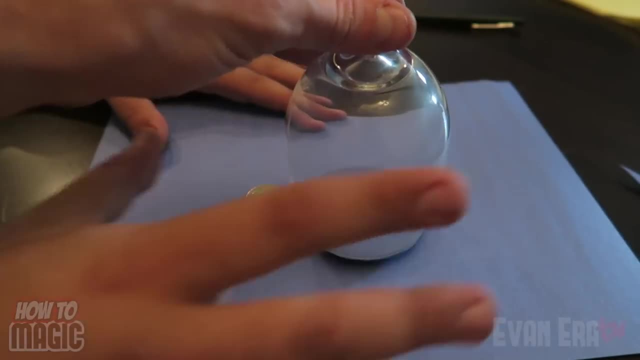 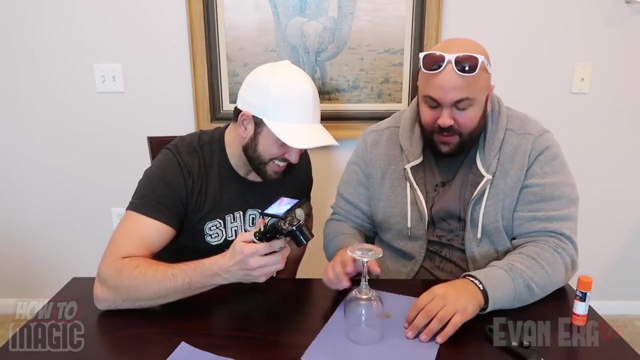 This is a cool one dude. Look at that. So you can like put your hand over it to block it or put a sash over it. Oh, that's cool. All right, I like that one dude. So this is like super simple and you can instantly repeat it for people. 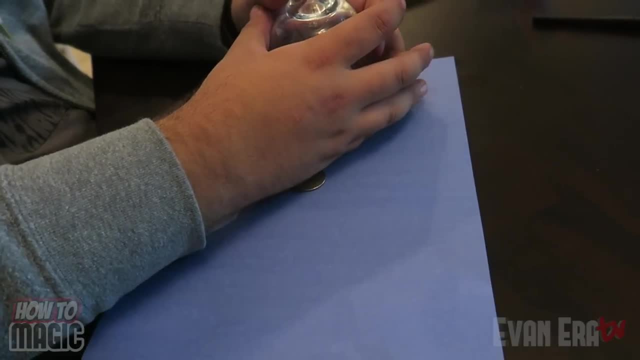 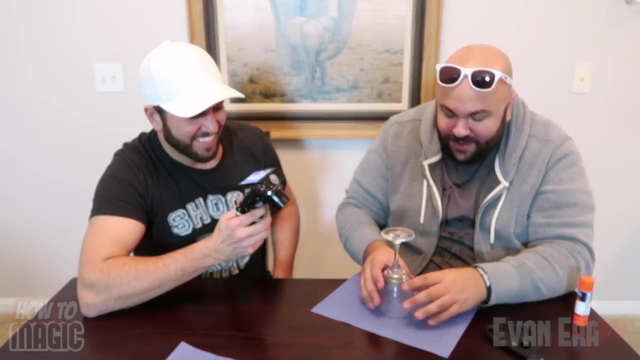 So you have the coin there. I like to like put my hands in front of it to kind of shield what they're seeing. I scoot it over and then it's gone. Wow Right, That's awesome. You can make it come back by just reversing the process. 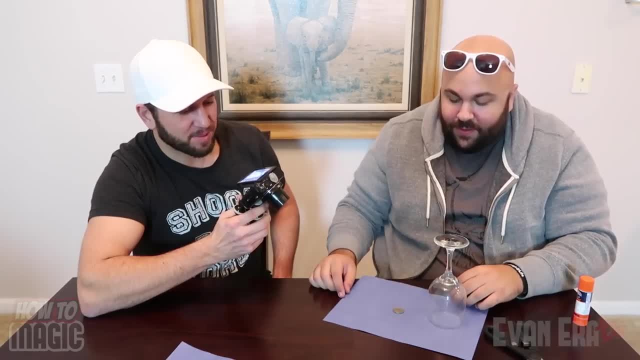 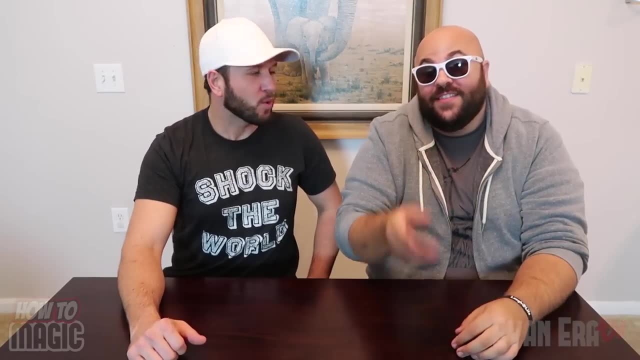 There it is. Boom. That's a good one. I like this one, And that is how you do the magic disappearing coin trick. Okay, this one is a cool magic trick that you can do with school supplies. Let's check it out. 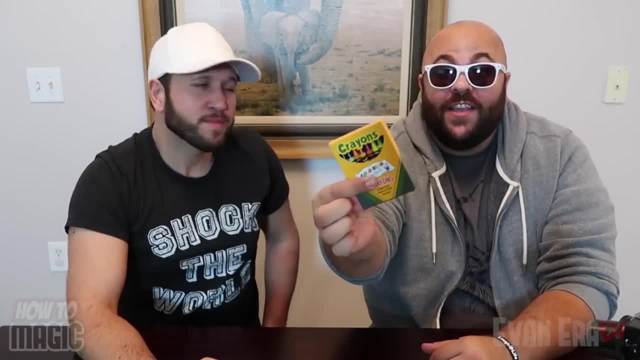 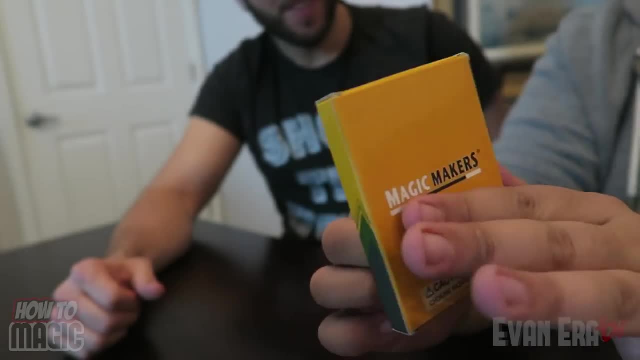 Okay, so you're going to take a box of crayons, present them to your audience, Call attention to the crayons and tell them to watch. As you wave your hand, the crayons just magically disappear. Can you bring them back? 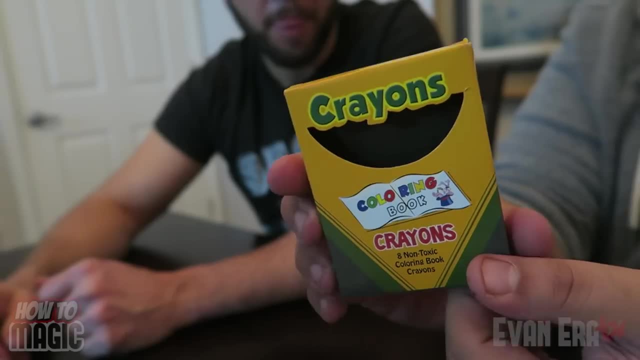 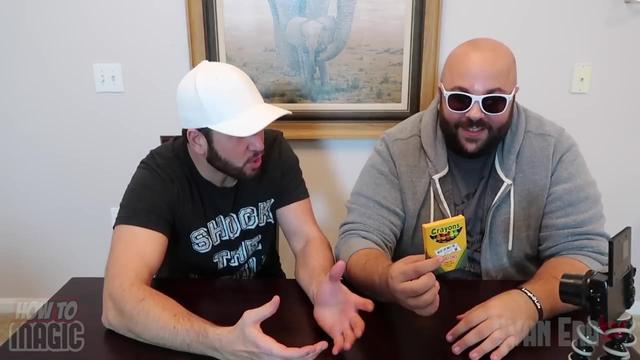 I can bring them back actually Watch. So in order to make the crayons come back, we just flip the box back this way and the crayons come back. That is so cool. How are you doing it? It's really easy. 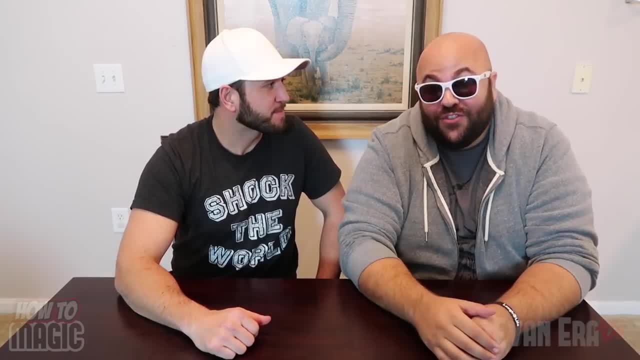 I'll teach you how it's done right now. Okay, here is the secret behind this trick. Okay, so this is a special box of crayons, not a normal box of crayons, And the real secret thing about it is how I'm holding it. 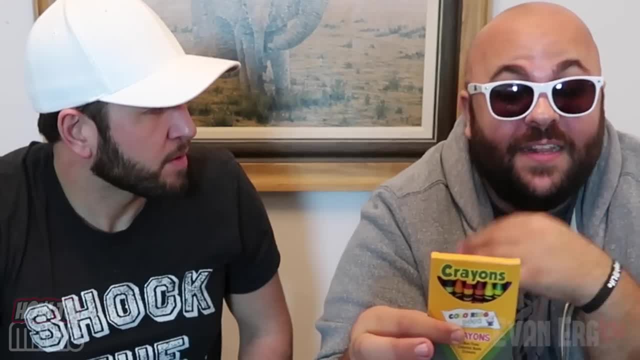 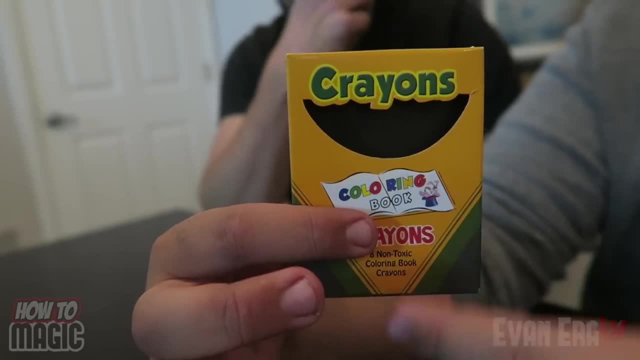 As I'm holding this pressure with my fingers, the crayons are in place, but as I lift the pressure off my fingers, watch what happens. The crayons drop down inside the box, hiding them from view and making it look like they completely disappeared. 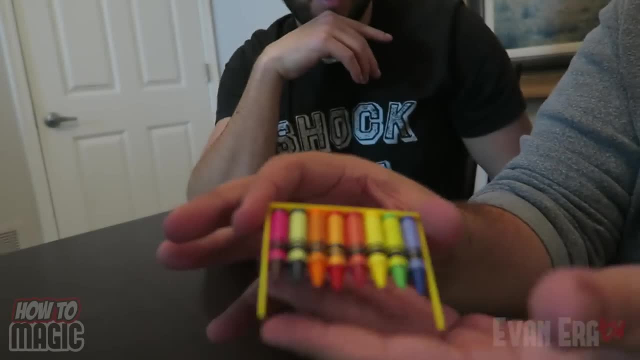 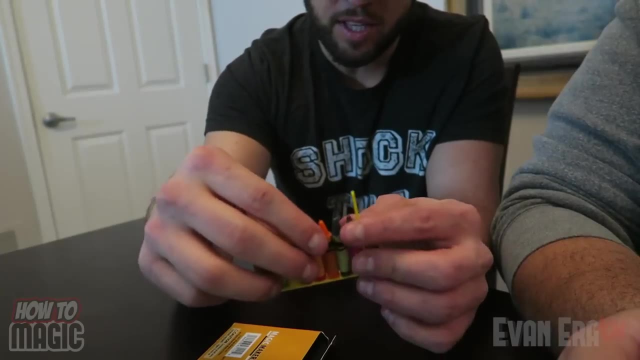 Now, if you open this up, I'll show you how this works. It's actually just like half of crayons, So you could theoretically make this at home if you wanted to. You're just going to cut your crayons in half. You could take a popsicle stick and glue them all on there. 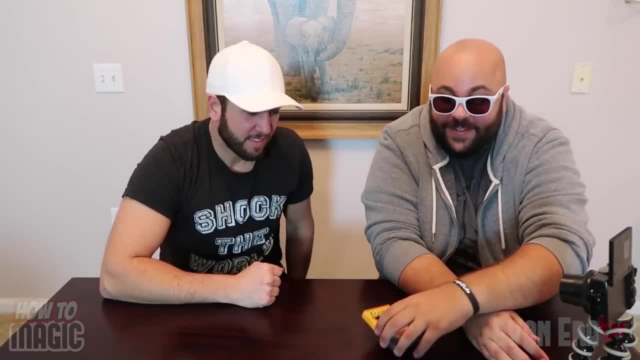 This would be a perfect one to take to school and show your friends. Totally easy to do and it looks really cool. So that's how you do the magic disappearing crayons trick. It's cold. It is cold out there, isn't it? 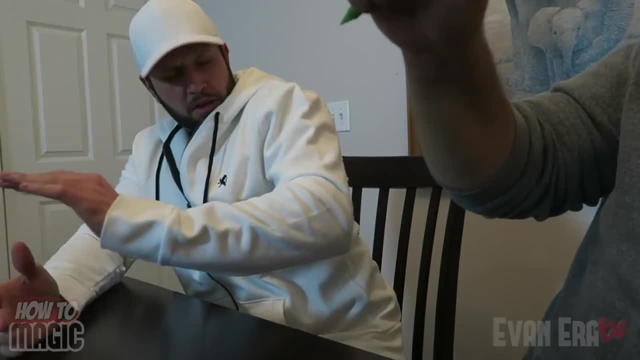 That's the next one. Are you ready? Yep, Let's do it. My mouth, bro. It's supposed to go on the shirt. This is the disappearing ink trick. Don't worry, It's not intoxic. So this is how it works. 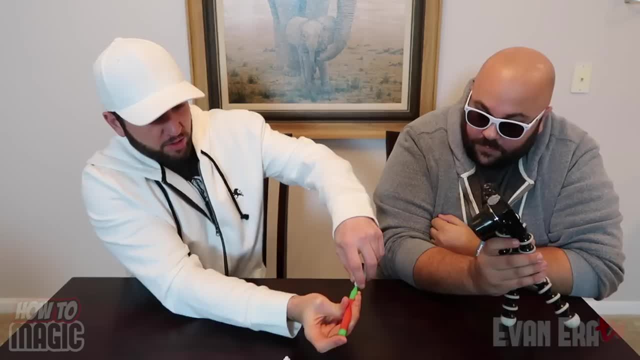 I fill it up through the tip of the pen And remember gravity. Remember gravity. The liquid will be down towards the tip. So when you go to make your squirt, make sure it's facing down. Don't come out on like a knife where it's up. 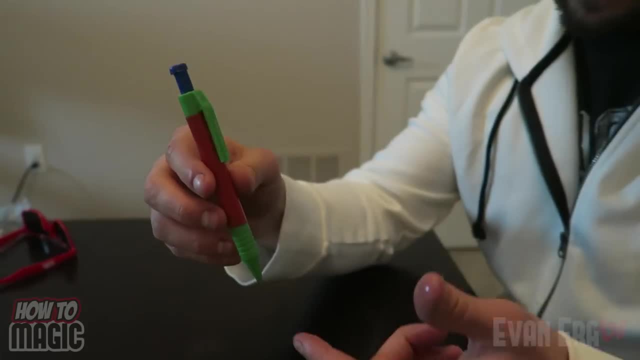 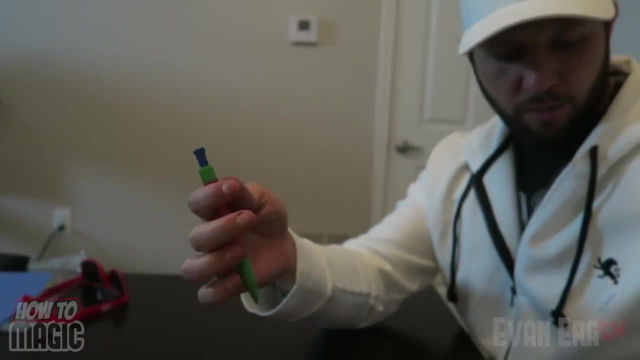 That's how you do it. Oh my goodness, Oh, no, No. So the idea is: oh my God, my shirt is ruined. No, It looks bad. It's so bad, dude, This shirt cost me $500.. 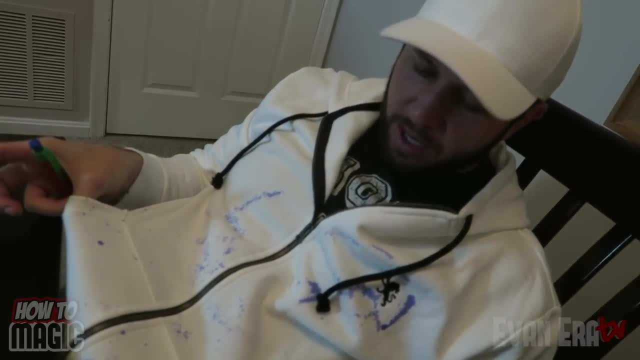 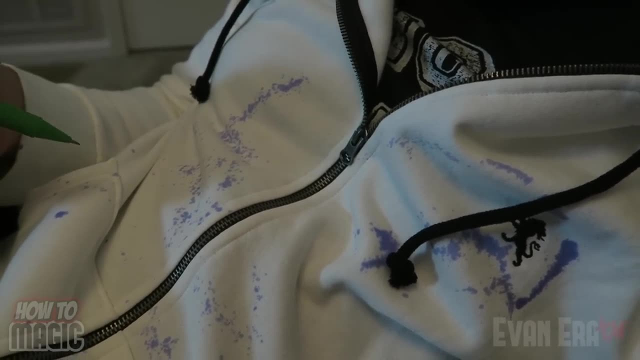 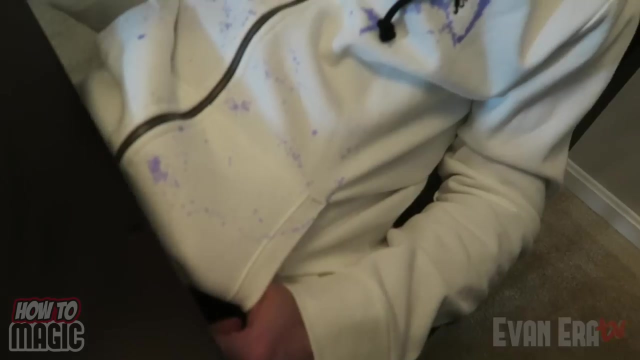 But then in five minutes, in like five minutes time, the ink will actually disappear. Awesome, It really gets a good reaction out of people. I'm sure it does, Because even though you tell them it disappears, it takes like five minutes for the ink to 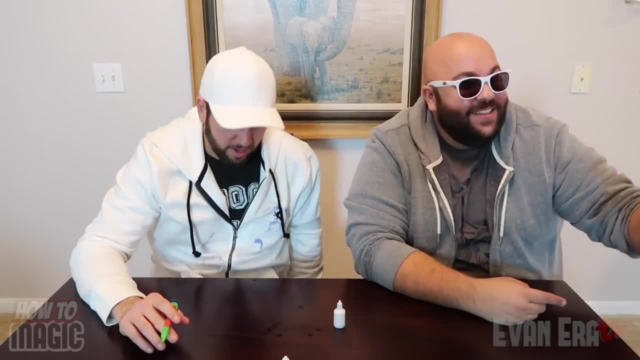 disappear And they really doubt it. If you don't know them, they're going to make you stick around for a while. It's just a vial of magic disappearing ink and you just pour it in the pen. It's pretty simple. 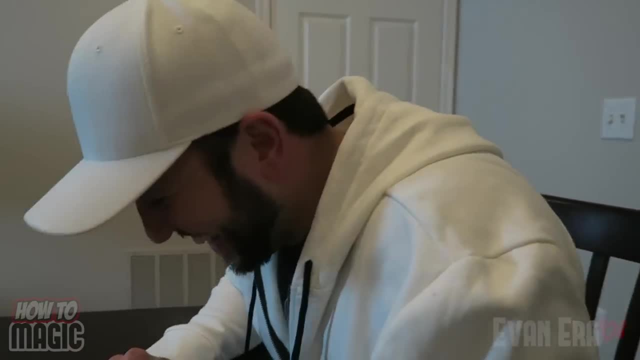 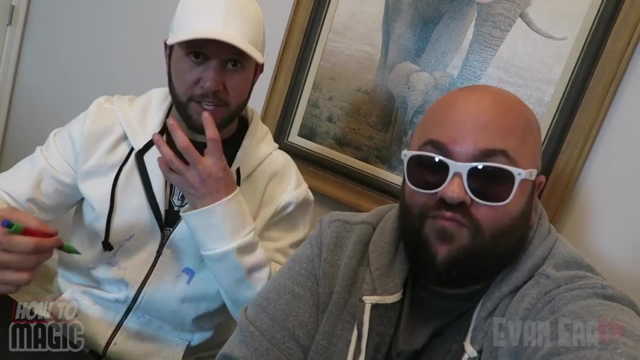 That's the simplest secret I've ever heard in my life. I told you it was easy. That's perfect, dude. That was the magic squirting ink pen trick. Remember? squirt it on the shirts, not in the face, Right. 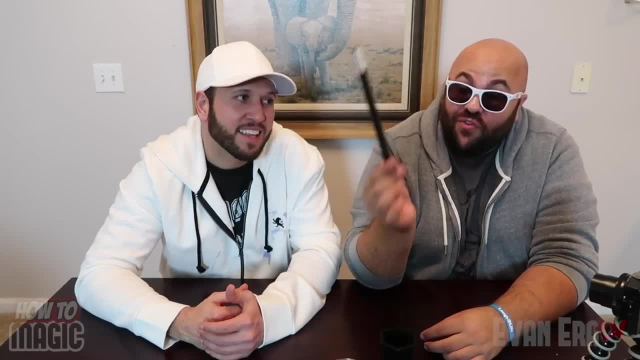 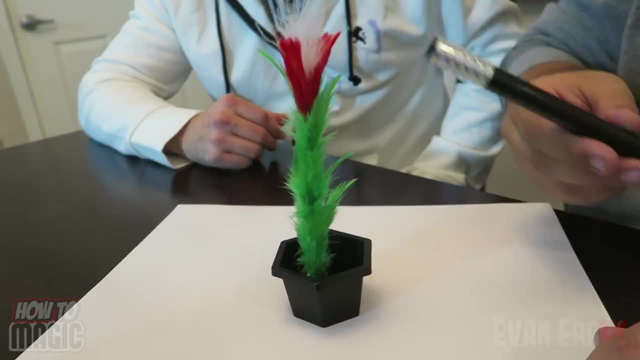 Yeah, Okay. So for this trick, you're going to do something really cool with a magic wand. Let's check it out, All right, So I'm going to take my magic wand and watch. Whoa, That's awesome. That's a little flower. 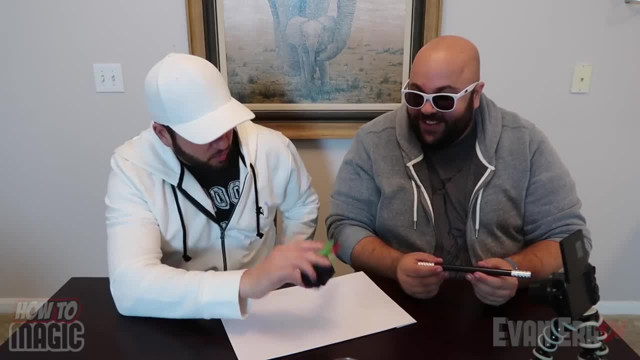 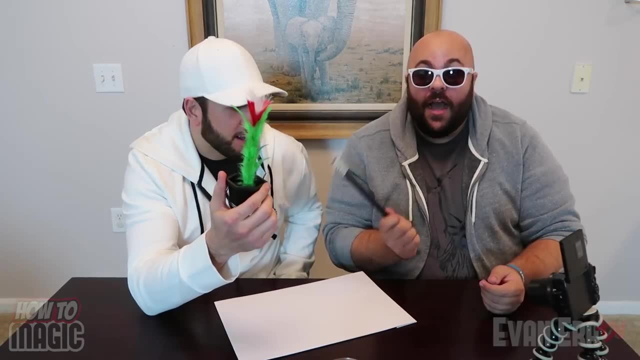 Right What It grew? It magically grew out of the pot. How, How, How. You want to learn how it's done? Yeah, I'll teach you how it's done. All right, Here's the secret, guys. 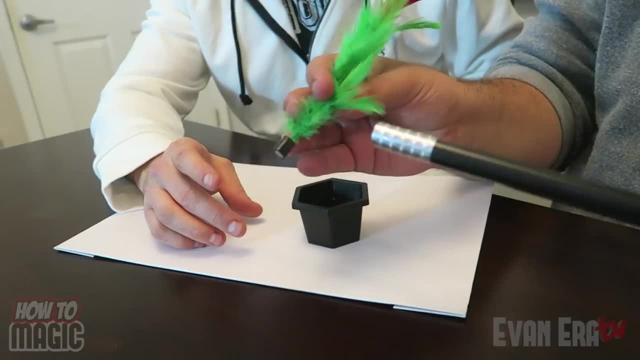 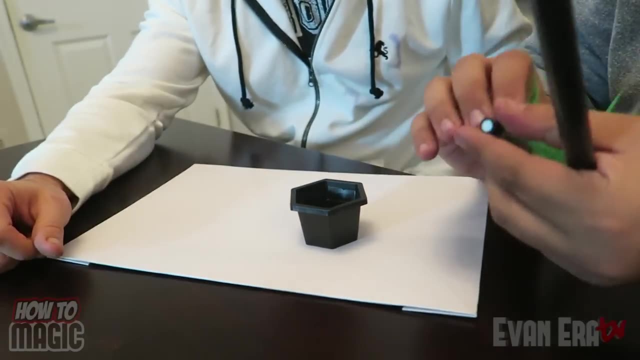 So this is a specially made magic wand and this little flower- it's like a feather flower. It's got a little magnet on the bottom. That's like the major secret to this trick. There's a magnet here and there's also a magnet in the base of this little flower. 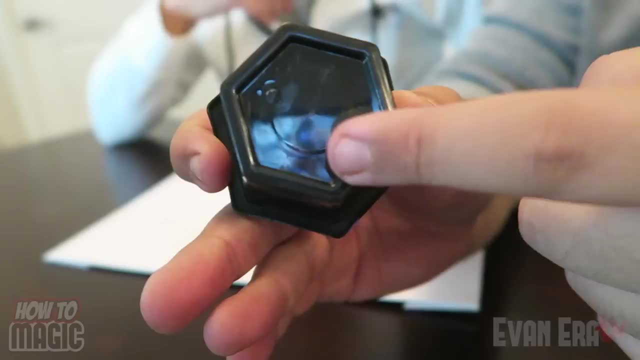 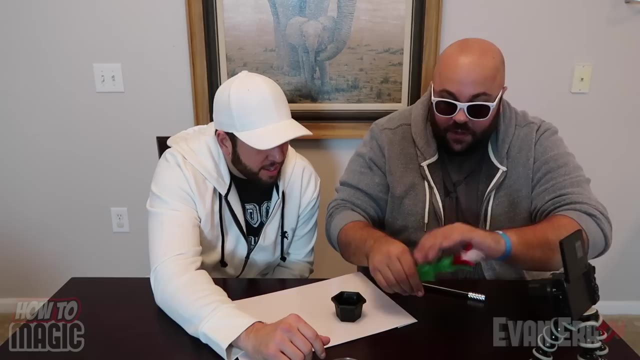 It's a little cup. So hidden inside the plastic of this cup, in the base of it, there's a little magnet. Look at that. Yeah, It'll stick right there. So the reason that's important is because this little feather flower goes inside your. 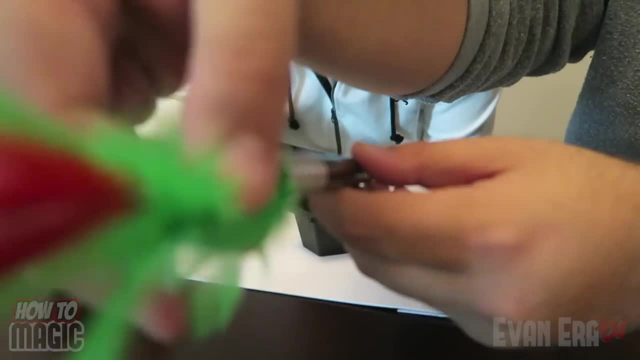 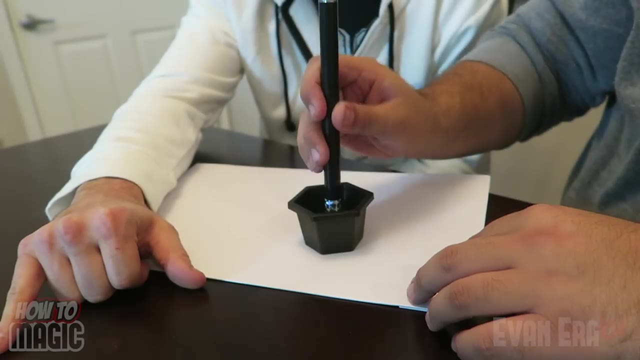 magic wand. This wand is hollow. This goes inside the magic wand like that. It's hidden inside so that the tip of the magnet is right at the end of the wand, so that when you touch it to the base, the magnet sticks. Whoa. 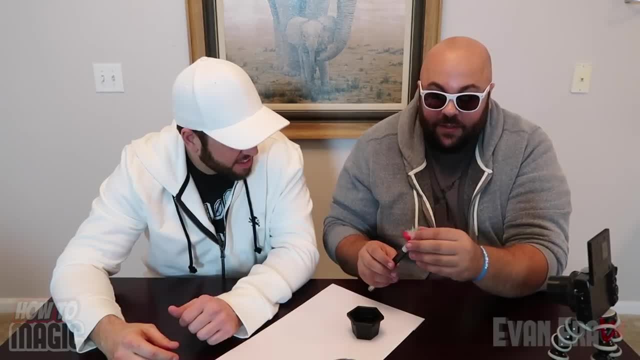 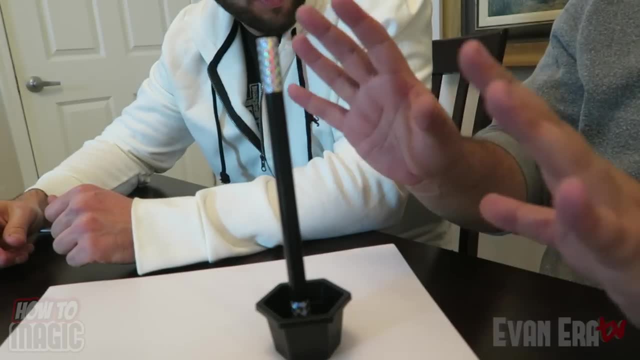 There you go, the flower. I love this one dude. Cool right. You kind of make this like a whole routine. You just take your magic wand and sit it here and be like watch. I can make my wand magically stand upright without touching it. 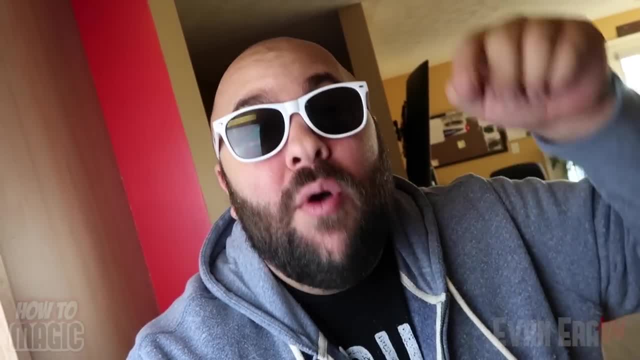 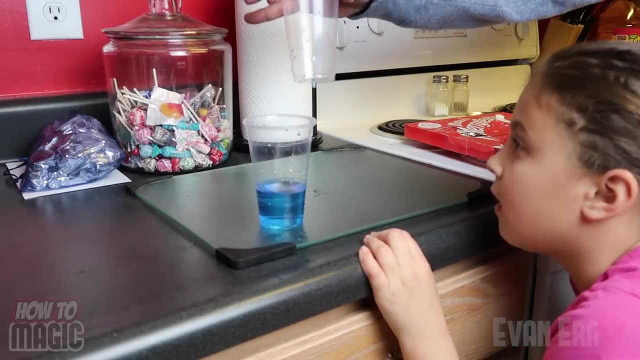 And then produce the flower. Okay, this is a super easy one you can do at home right now. This is the liquid through the cup trick. Okay, watch One, two, three. Look. How did you do that, Dad? 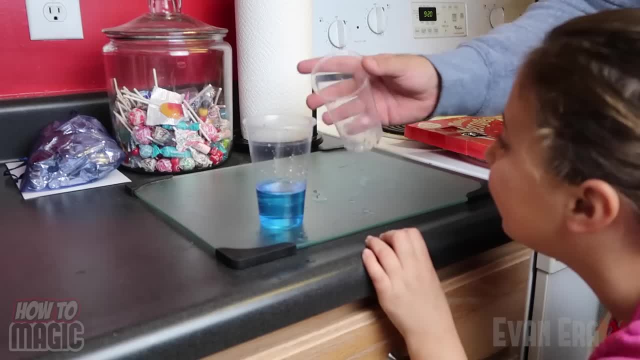 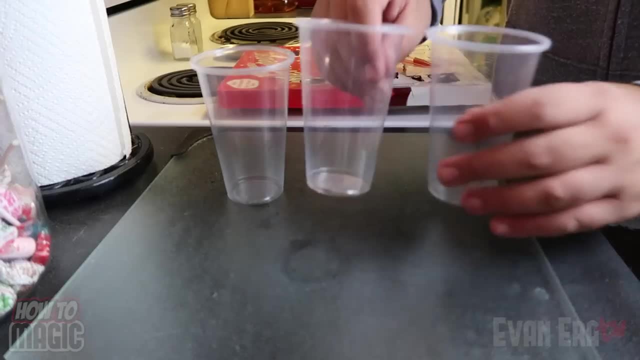 Cool right, And the liquid goes right through the cup. The secret to the trick is extremely simple, and I'll teach you how it's done right now. All right guys. so really simple explanation to this trick. All you need to do it are three plastic cups. 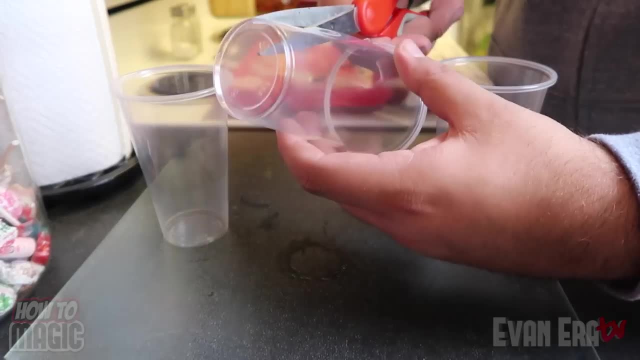 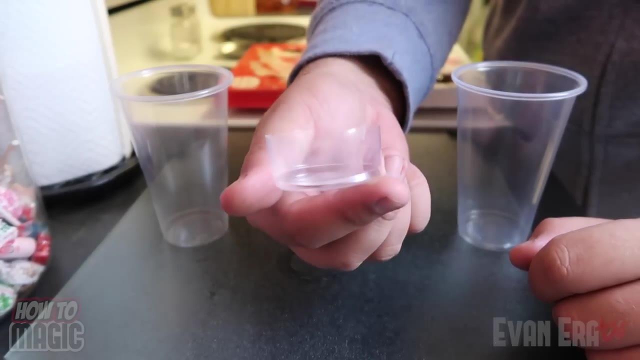 They need to be clear cups. You're going to take one and you're going to cut down the side, just like this, and around the bottom, so that you're left with this right here about an inch long bottom of a cup, And you're going to take that and fill it with some of your blue liquid. 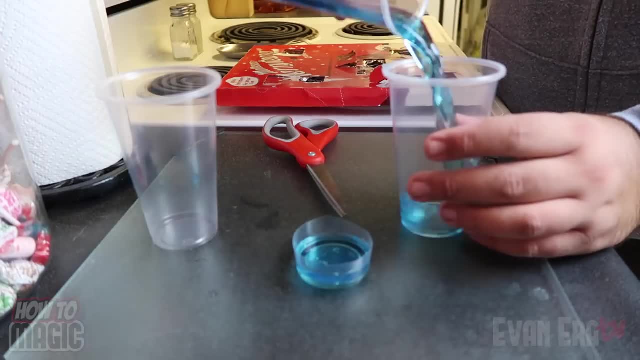 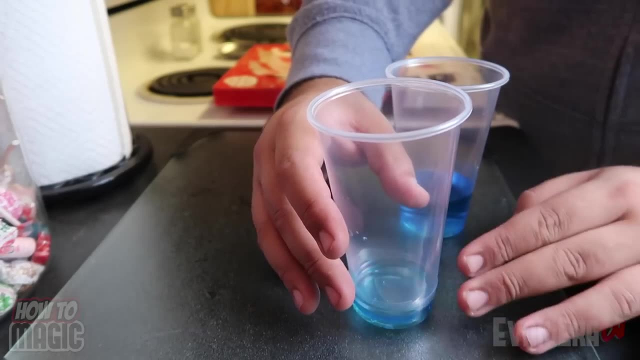 This is just water and blue food coloring. You're then going to take your other cup and fill that with blue liquid. Now, here is the secret: You're going to take the little bottom of the cup and you're going to put your other cup inside it. 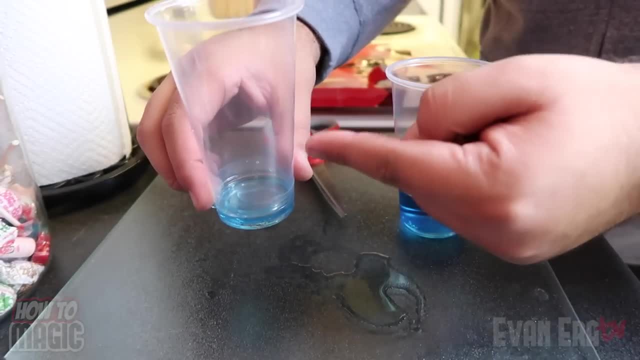 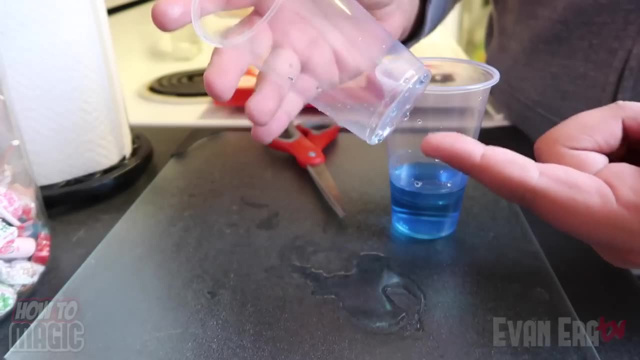 And now it looks like you have a little bit of blue liquid in the bottom of this cup. So when you come over here, just drop it in The bottom of the cup will drop into this cup and disappear into the liquid, making it look like the liquid in this cup just penetrated through the bottom of the cup into that one. 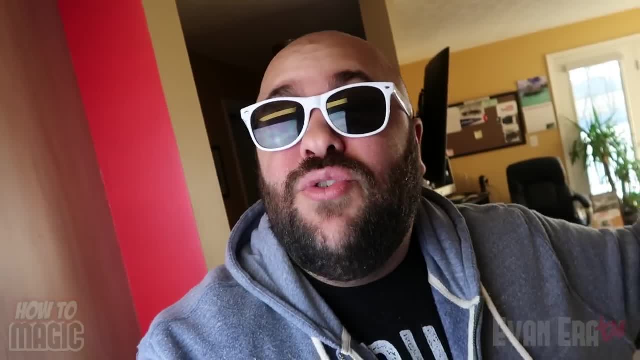 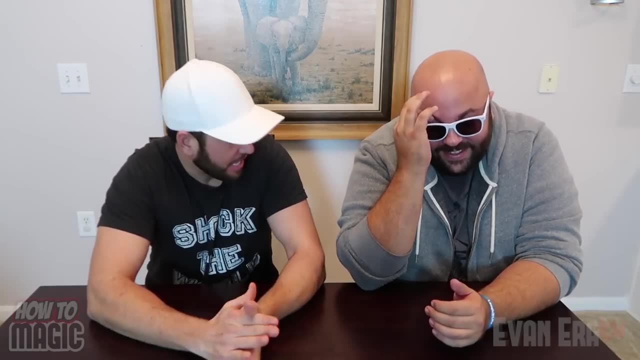 Super easy to do. Try it at home and let me know your results. And that is how you do the magic liquid through the cup trick. Woo, That was good man, That was fun. Those magic tricks were easy, So we got the outro next and that's it. 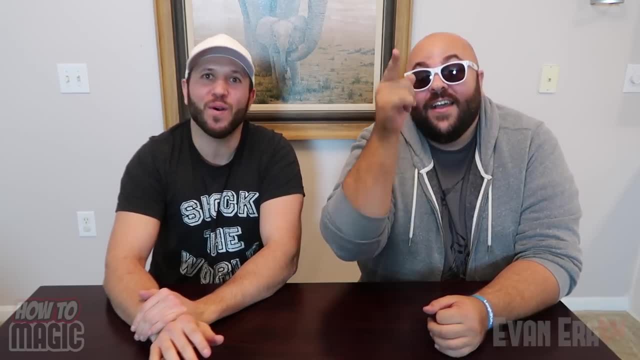 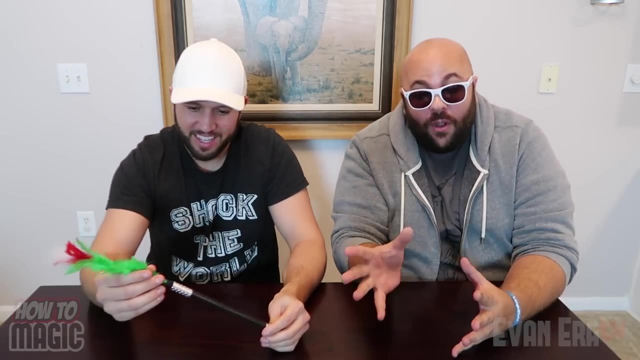 It's actually giveaway time. Ooh, Yes, Guys, it is giveaway time. I'm giving away all the props from this video. All of them, All of them. No, The magic appearing flower Dude- this is my favorite. 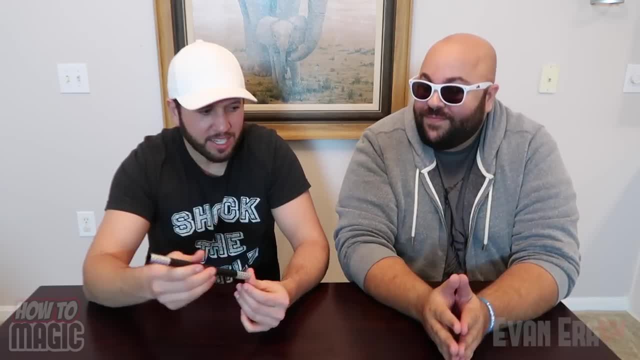 The disappearing box of crayons, The magic ink squirting pen- Well, actually I take that back. I like the crayon one better Crayon one's your favorite? Yeah, this is my favorite because I could just do it over and over and over and be fun. 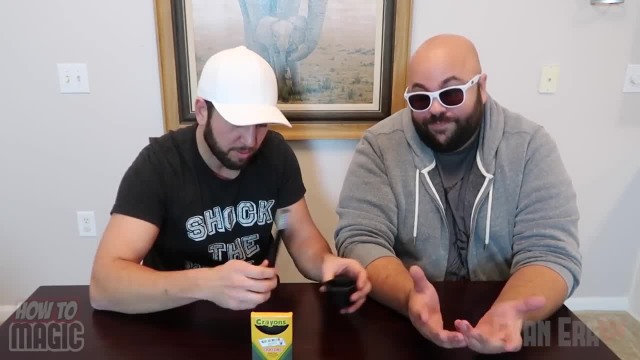 Right, This is my pocket, This one's big. I got two pieces, Three pieces. Wait, You're going to give away my wine glass, bro, I'm not giving away my wine glass. You're going to send my wine glass away to someone who breaks? 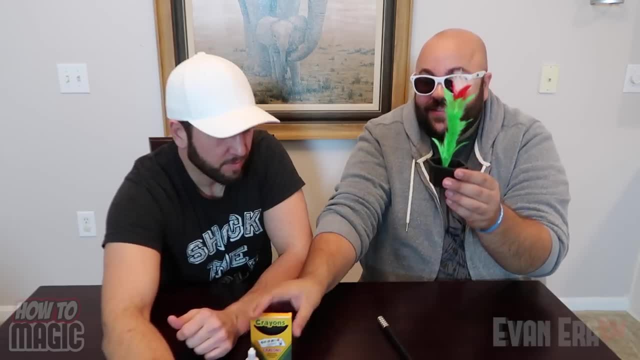 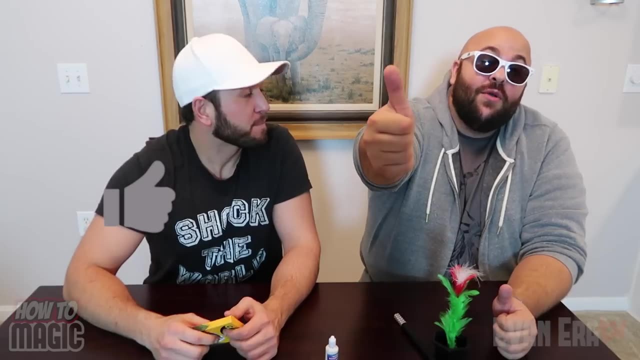 You can do that one at home. All the props from the video like this, this one magic ink pen- all of them are up for grabs in the giveaway. All you got to do to win one of these items: give this video a thumbs up. leave a comment. 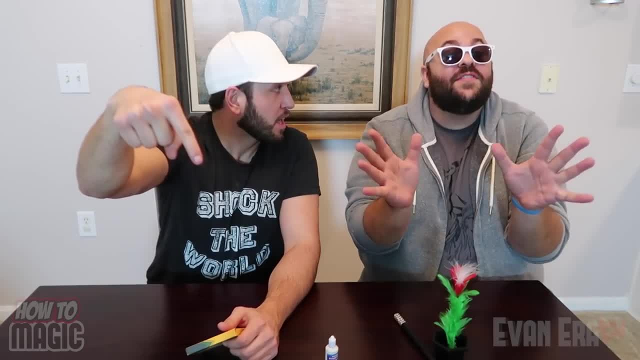 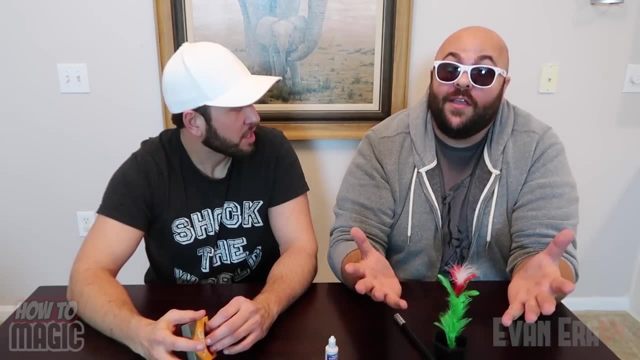 in the comment section below. That's it. That's all you got to do. You can leave as many comments as you want. What do they got to comment? Whatever you want, Leave something funny, Something like What's a joke you can think of. 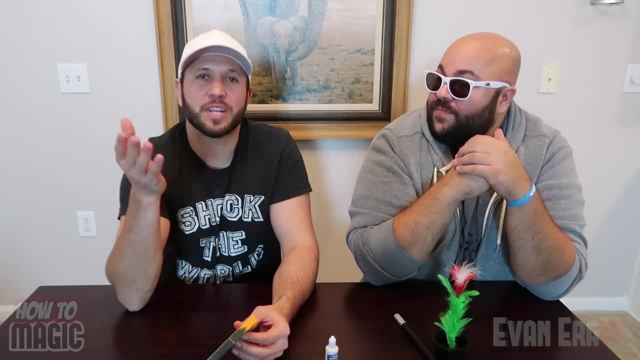 Leave a joke in the comment section below. Those are funny. I want to hear some jokes. If you can't find a joke or you can't think of a joke, go to Google and show the joke. Yeah, Leave a comment in the comment section on this video. 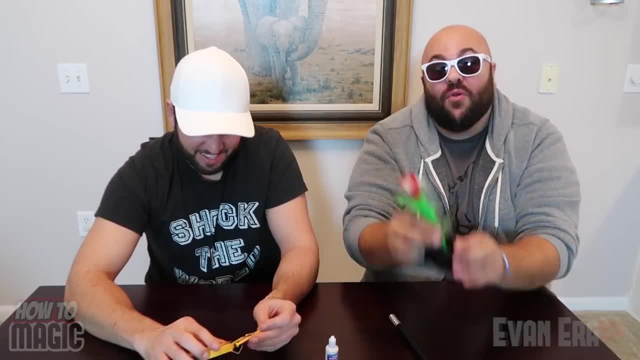 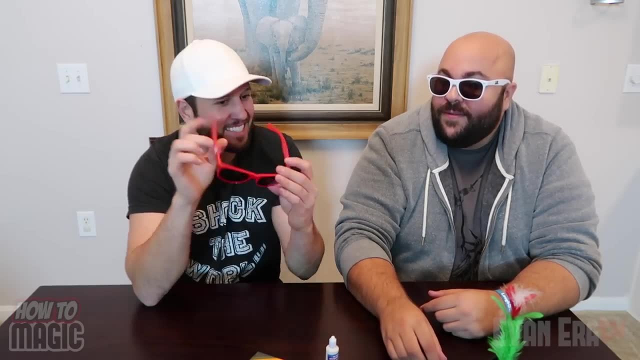 Give it a thumbs up. I will pick five random comments and I will mail you one of these props. Make sure they're funny jokes so I can laugh at life. I like that. Wait, Are you giving away this red pair of sunglasses? 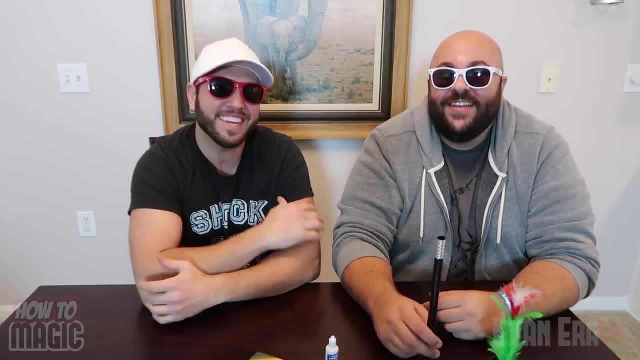 Sure, They weren't part of the props, but they were part of the video. You got to give away the red glasses too, because it's Christmas time. I got red and green glasses. We're giving away One pair of red, one pair of green. 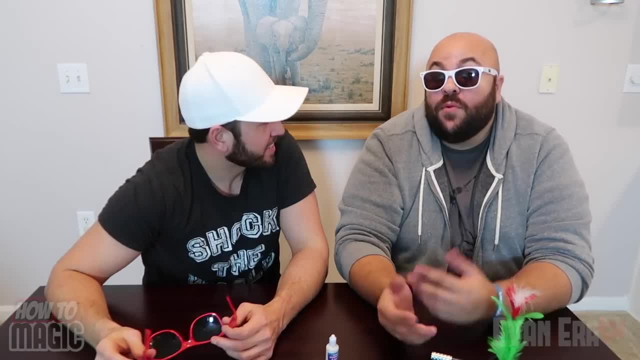 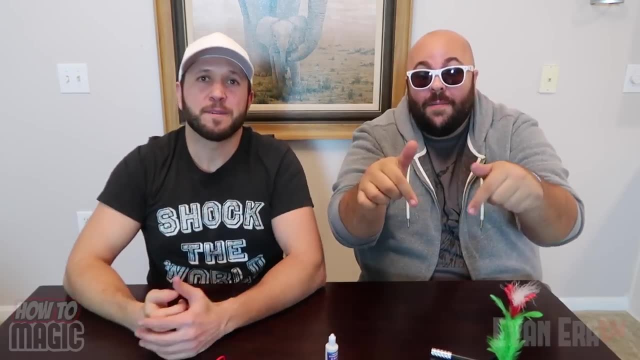 Thumbs up Comment. Funny joke. You can Share it on your Facebook or Twitter Text or email it to a friend. You know what to do. If you're new to the channel, be sure to subscribe. If you're coming over from Dennis' channel, be sure to subscribe. 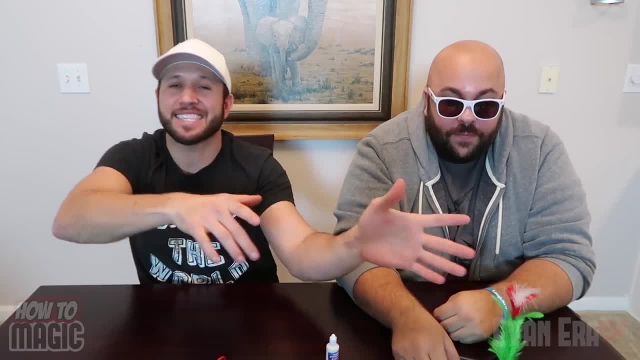 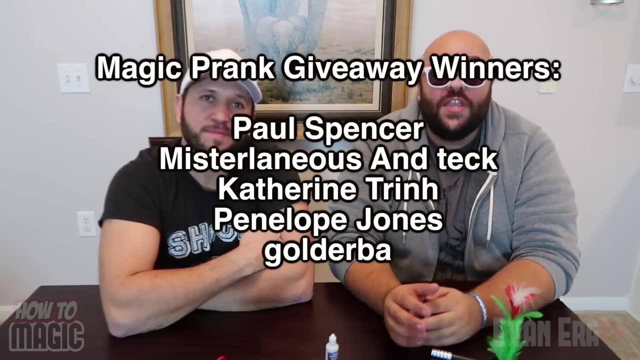 Hit that bell so you get the notification, and then tap the links at the end. whichever way, they're going to come in for more how-to pranks. All right, guys, It's time to announce the giveaway winners from the last How To Magic video. 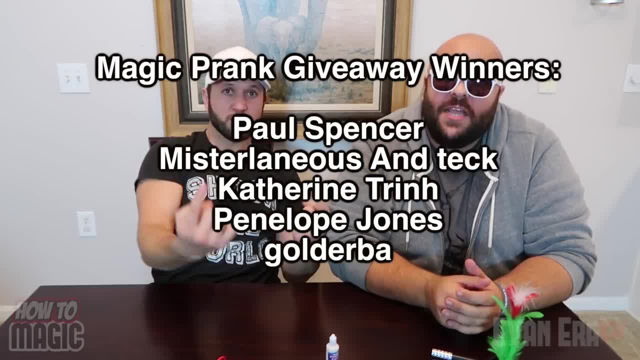 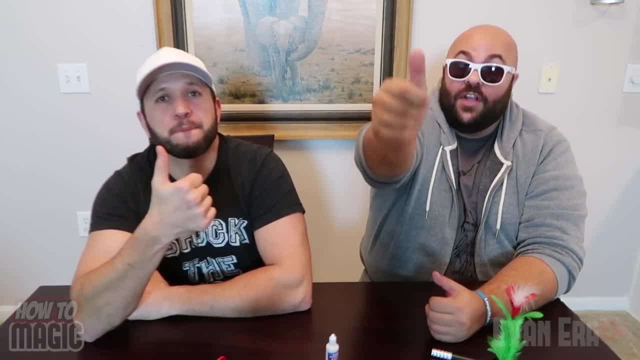 The winners are these names right here. Send me a message on YouTube to claim your prize. Thank you to everyone who entered the giveaway drawing. Good luck And good luck to everyone entering this giveaway drawing. Be sure to give the video a thumbs up and leave a comment below. 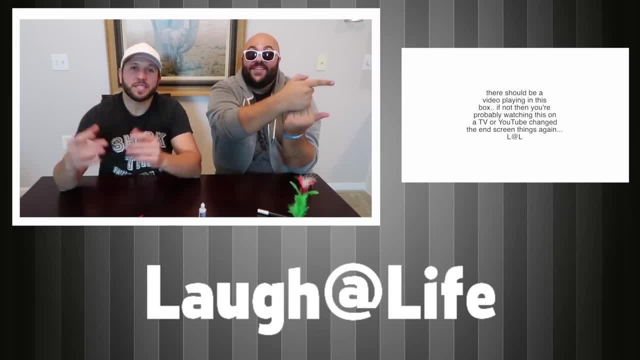 All right guys, Be sure to click the video right over here that we did on Dennis' channel. We did gift wrap pranks- perfect timing for Christmas, Don't miss it. So go check out Dennis' channel, Go subscribe to How To Prank It Up. 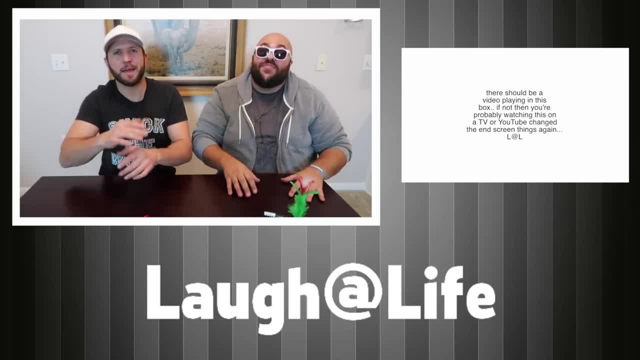 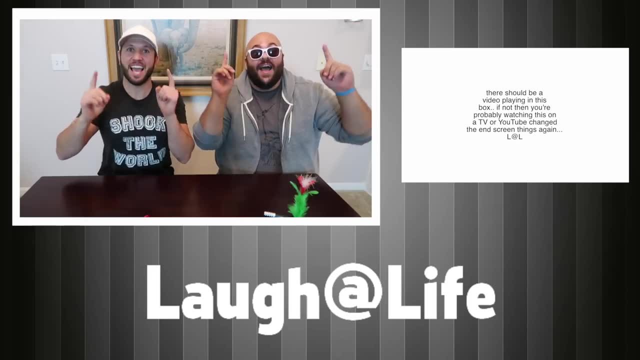 Make sure you leave a comment. Let me know you're from the Era Squad. Until next time, thank you for coming back to Evanera TV, where anything is possible as long as you stay positive, work hard and laugh at life. Love you guys.